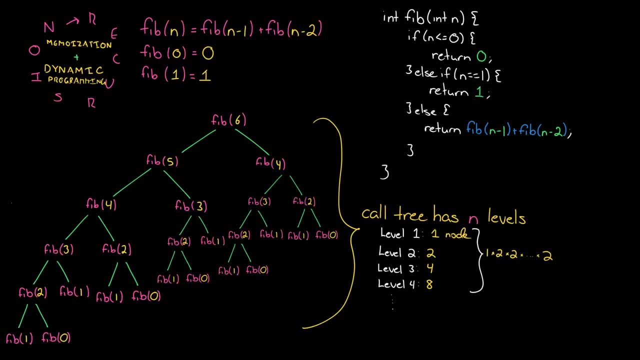 So if you take one, you double it n times because we have double the number of nodes at every single level. we're going to wind up with roughly 2 to the n nodes in the tree. So this goes up for us a runtime of 0 to the n And if you remember, I was able to compute this by hand. 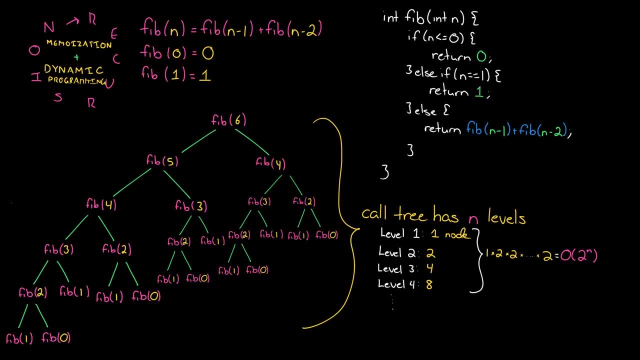 fairly quickly, And so there's a bit of a mismatch here. Why is this algorithm so inefficient? And the reason is that we keep doing things repeatedly. We compute fib of 4 twice here and here. Fib of 3 gets computed three times here, here and here Fib of 2 gets. 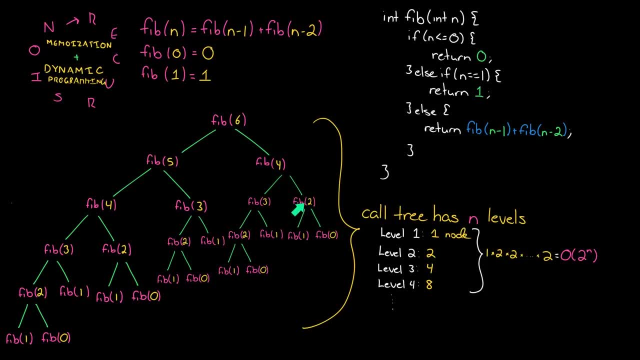 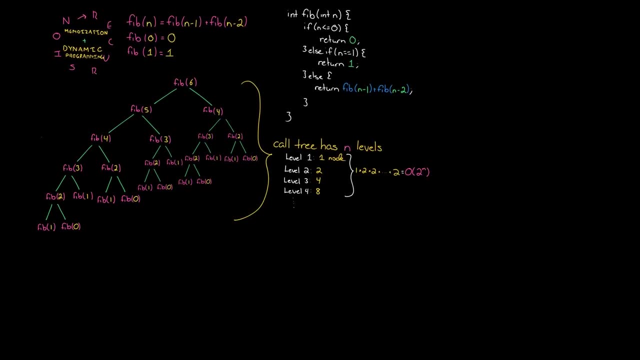 computed five times here, here, here, here and here Now. obviously, these values have changed. Fib of 4 is always the same thing, Fib of 3 is always the same thing. So what we should be able to do is just compute these values once And, if we ever have to compute them again, 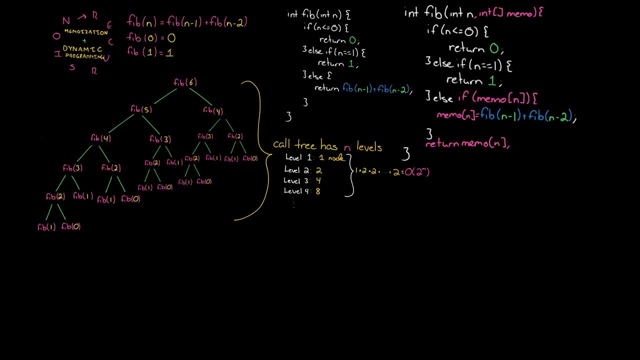 just return the stored value. So we store the value each time rather than computing it from scratch, And that's what the most basic implementation of a memoization algorithm is. So now, if we walk through what this code does, we're still going to go. 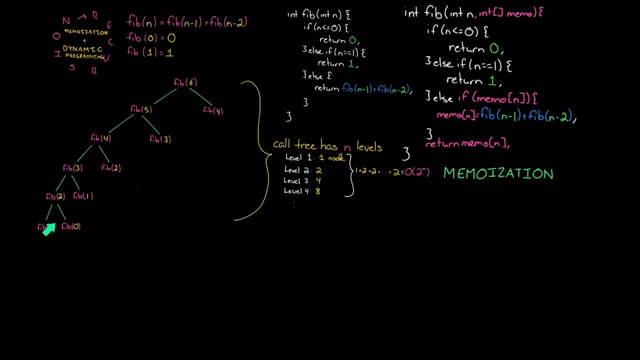 and compute this whole path down here. But when we do that, we're going to build up this table. So then, when we get down to computing fib of 1, well, that's a base case. Fib of 2, hey. 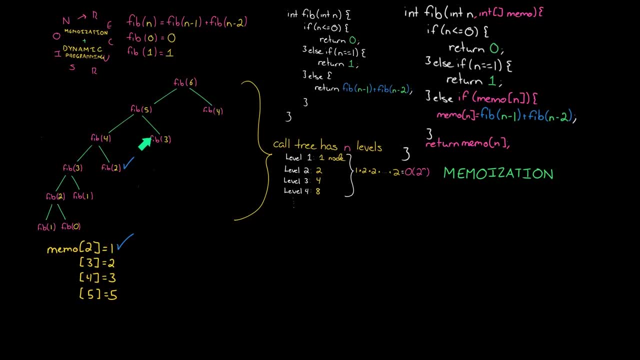 already been computed. We just return that value- Fib of 3, already computed, Fib of 4, already computed. So, although we still recurse just as deeply, all our other work has been done by that point and we're just returning stored values And now we get a linear runtime instead. 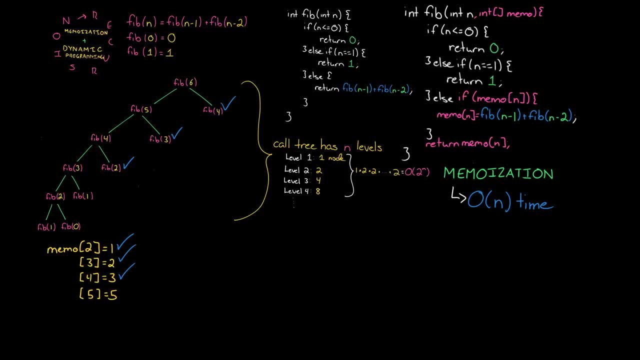 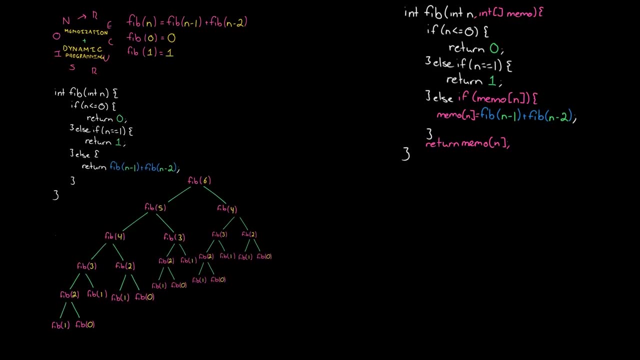 of exponential, which is, of course, an enormous improvement. So now let's talk about space complexity. Space complexity comes from any memory that we have, Any memory you use, And that includes, yes, things like creating arrays and stuff like that. 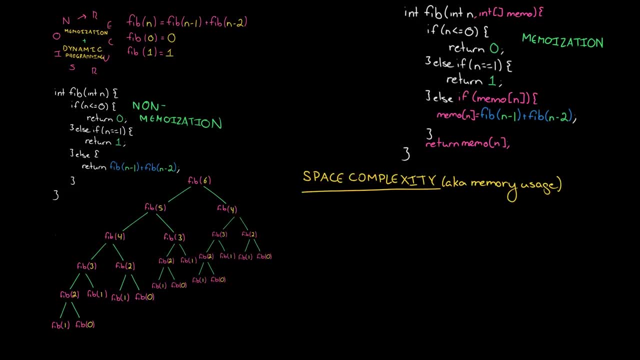 but it also includes the call stack. So let's think about the space complexity of the non-memoized solution. A lot of times people will describe this as O of 2 to the n, and that's actually a mistake. People are thinking: well, gee, all O of 2 to the n, things are all in the call stack. 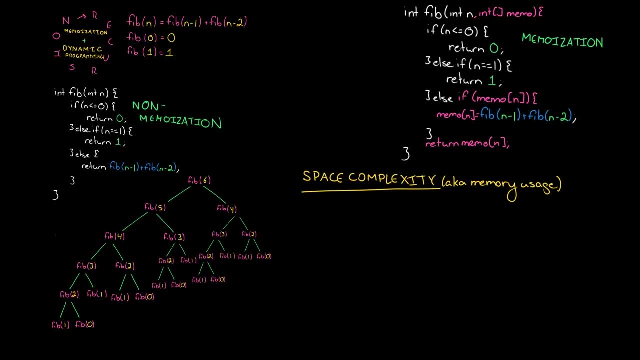 so we need all of that? Yes, but they're not all on the call stack at the same time. One way to think about space complexity is: if I were to give you a chunk of memory to run your program, how big would that chunk of memory have to be? 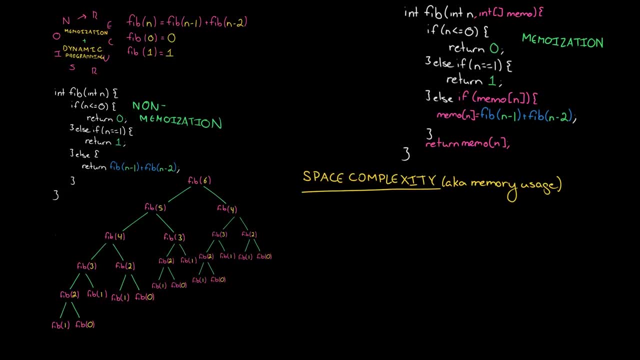 Although all O of 2 to the n things wind up on the call stack over all time, they're not all sitting there at the same time. The biggest your call stack ever gets the most memory you have in use at any one point in time is O of n. There's only O of n things. 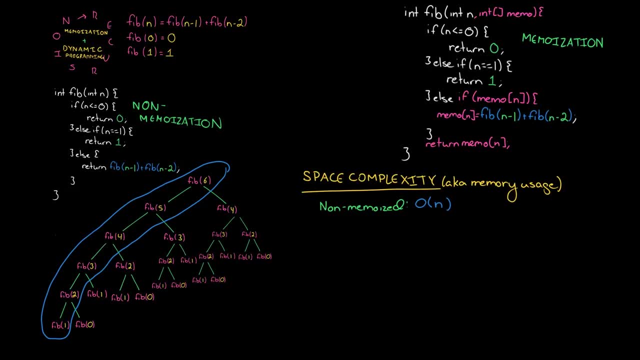 that wind up on the call stack at any one given time. So the space complexity of the non-memoized solution is O of n. The memoized solution also has their space complexity of O of n because we need O of n memory for the call stack still and we need another O of n memory. 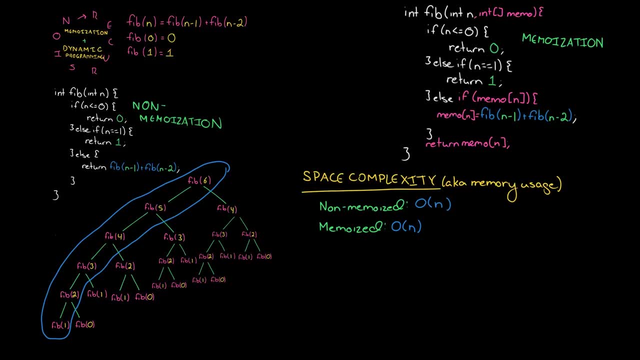 for the memo table. But O of n plus O of n is still O of n, So both of these have a space. complexity of O of n. Now let's try this out on a new problem. Suppose you're given an n by n grid. 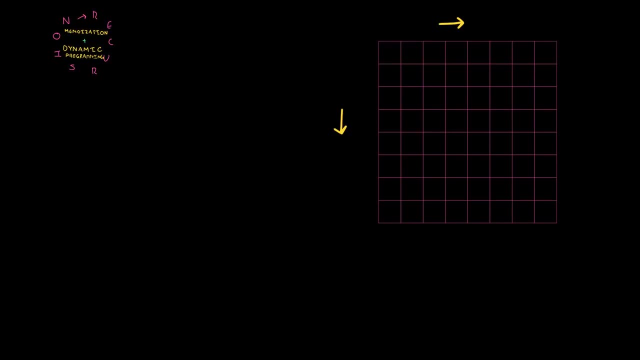 and you can only move down or to the right, and certain cells are blocked off in this grid. The question is: how many paths are there from the top left to the bottom right? As you might guess, we want to approach this recursively, So let's break this down into. 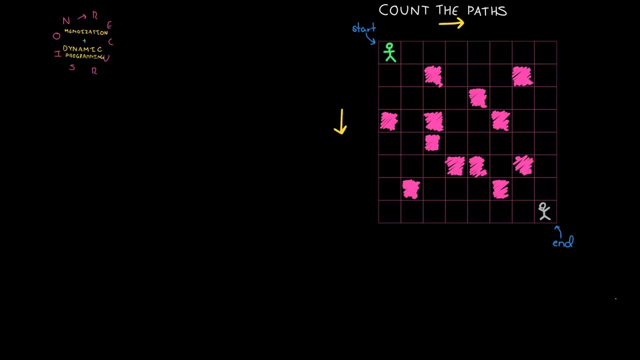 smaller problems. The overall problem is: how many paths are there from the top left to the bottom right? Well, let's think about this green guy in the top left corner. The first decision he needs to make is: well, am I going to go down or to the right? Those are my only options. So let's picture. 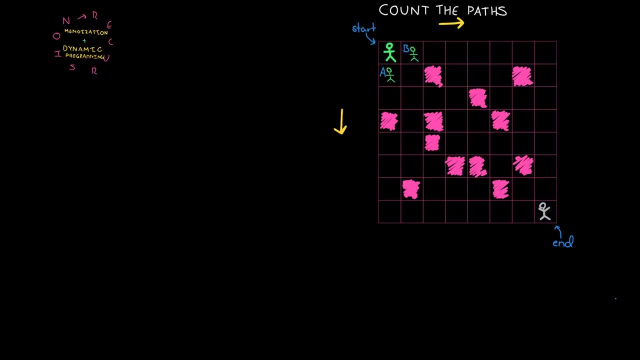 each of those options. There are only those two ways of going. So the number of paths from the start to the end is the number of paths from both sides of the grid And the number of paths from position A to the end, plus the number of paths from position B to the end. So now we've broken. 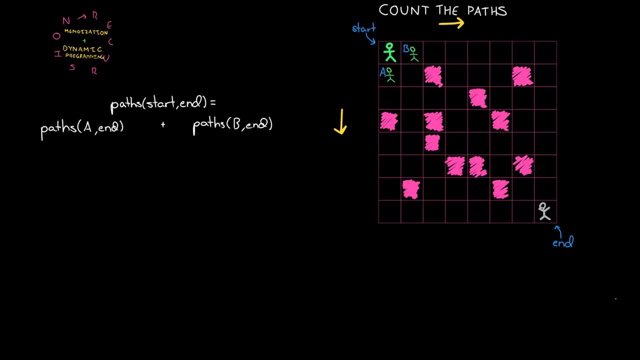 down our problem into other subproblems. So now what happens? Well, person A has to go either down or to the right. again Same with position B. So now the number of paths from A to the end can be broken down into C and D. It's the number of paths from C to the end plus the number of 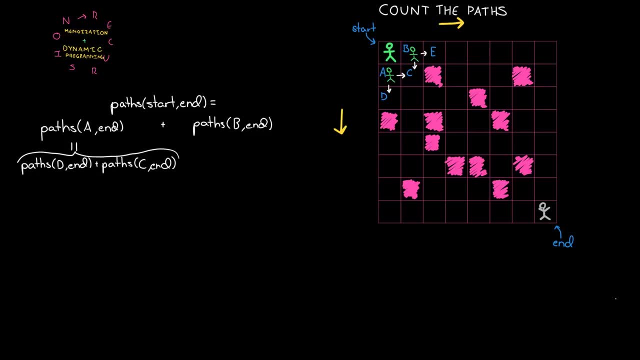 paths from D to the end. Same thing with B. It's the number of paths from B to the end. it's the the end plus number of paths from E to the end. This recursion stops when we have a definitive answer, and that comes when we're actually at the end. The 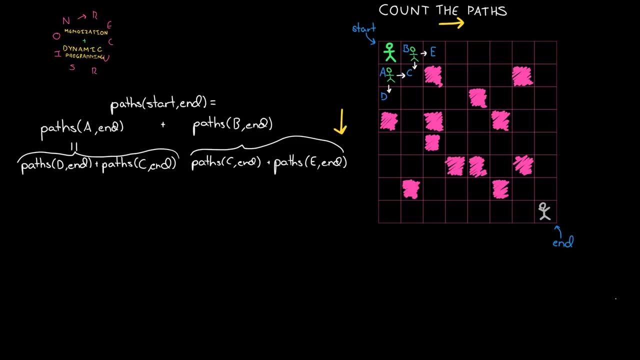 number of paths from the end to the end is just one. You stand exactly where you are, So that forms our recursion base cases. Translating this into code is relatively straightforward. We just traverse down and to the right, obviously making sure we check you know that we're not out of bounds or in a blocked off. 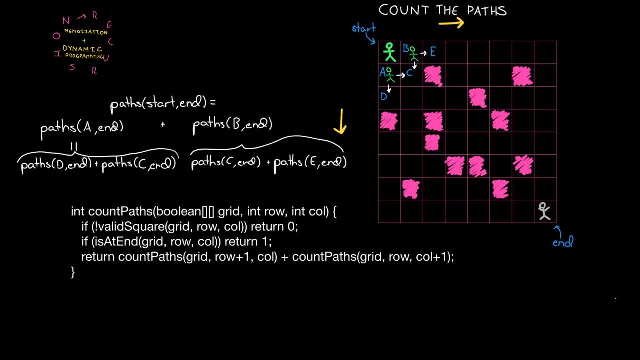 square, but then we just sum up the number of ways of going down plus number of ways of going to the right, And when we get down to the actual end we return one. This is a pretty straightforward implementation of that algorithm. ValidSquared does both the boundary checking as well as making sure we're 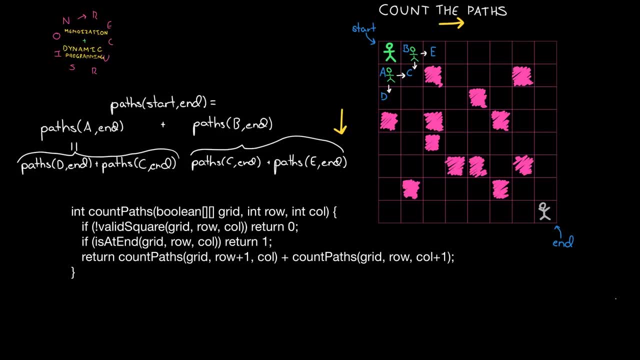 not in a blocked off square. If we are, then we turn zero because there's no paths. If we're at the end, return one, because there's just the one path. You stay right there. Otherwise, the number of paths from here to the end is the number. 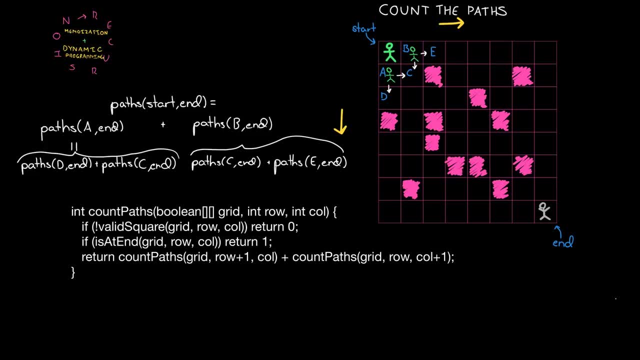 of paths going down to the end and the plus number of paths going right to the end. One little tip, by the way, was that if you're at the end, you don't have to go down to the end. You can just make sure you're at the breaking point and hit it. So it's basically going down. 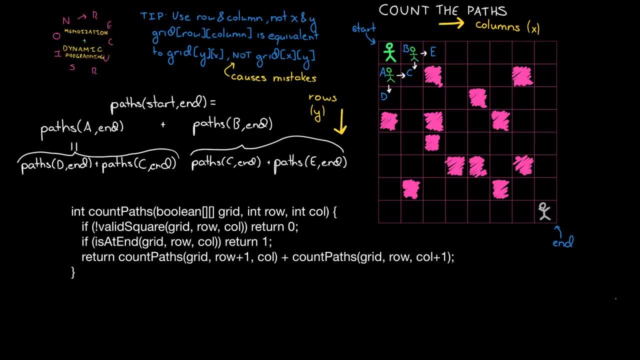 to the end, And then, if you're at the end, you go down to the end, You press one And then you just feel as if you're at the end, So that's the first thing that comes up. So this is actually all about the matrix problem. We have to get the matrix. 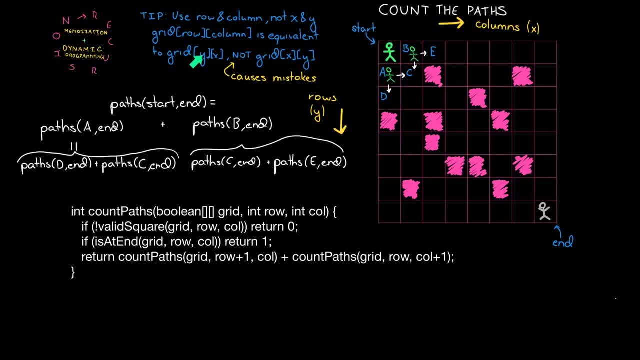 problem. right, Because the problem with matrix is. I'm an example of being able to write a matrix problem. So I'm going to write a matrix problem. And I'm going to write a matrix problem because when I do a matrix problem, I like to use row. 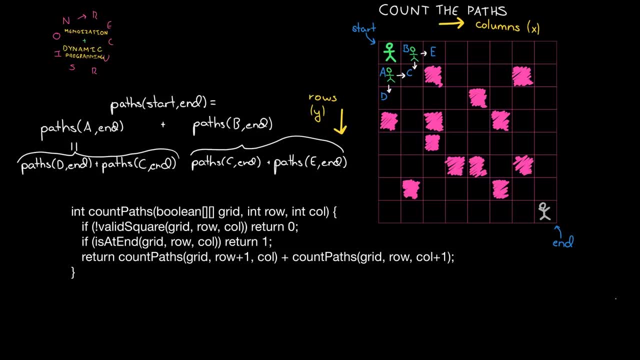 and column for my variable names, rather than X and Y, And the reason is that the above: we compute the number of paths from C to the end twice, And that's a necessary. What we should be doing is saying, hey, if I've already computed something, just return that stored value. 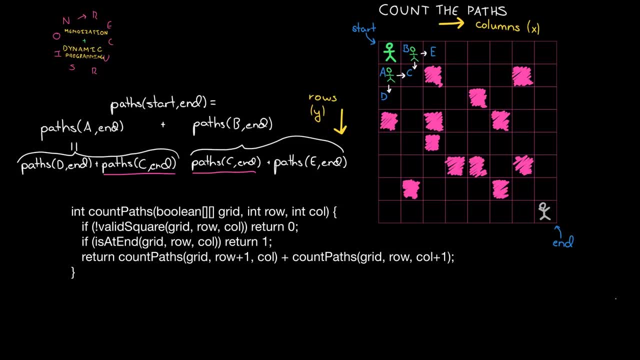 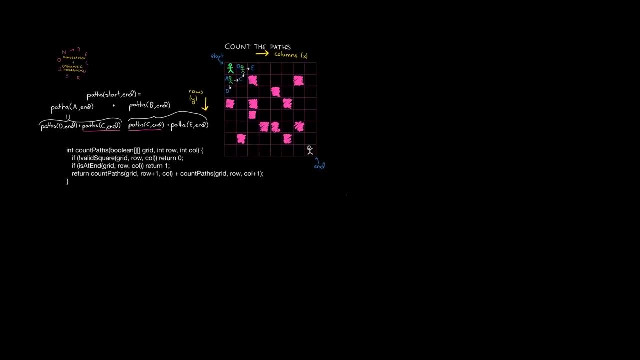 So every single thing I compute, I want to just store that value and return it if I ever ask for it again. And that's a memoization approach. Now, instead, we just compute it once and then, if we ever need that value again, just return that stored value, And that's all we have to do here. 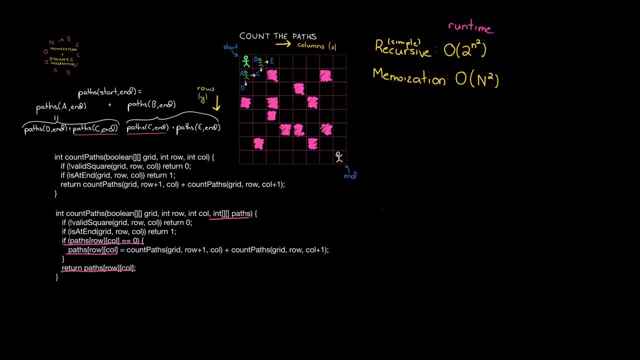 The runtime now is O of n squared, because we have n squared possible cells that we have to compute this for. But in each time we compute it it's constant time, given that we have other work already done. So that gives us a runtime of O of n squared. So if we want to, we can flip this around. 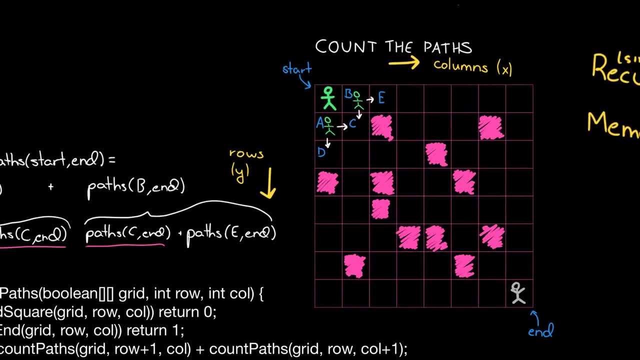 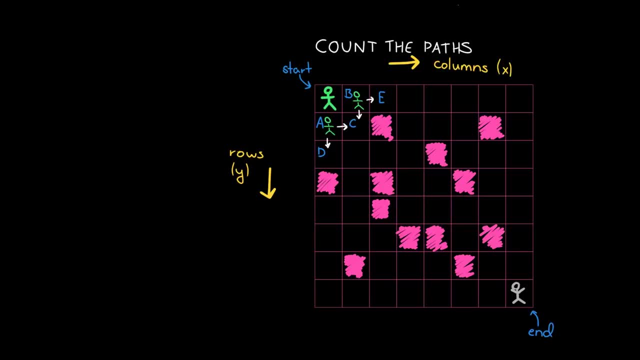 and do more of a traditional dynamic programming approach. So let's take a look at how this would work. If we think about what the recursive approach does, the very first concrete values it gets, other than the base cases, are these two, These two cells, And so that gives us two concrete answers. Now where can we go from here? 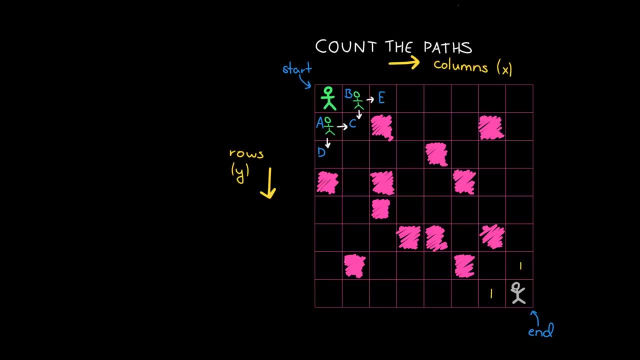 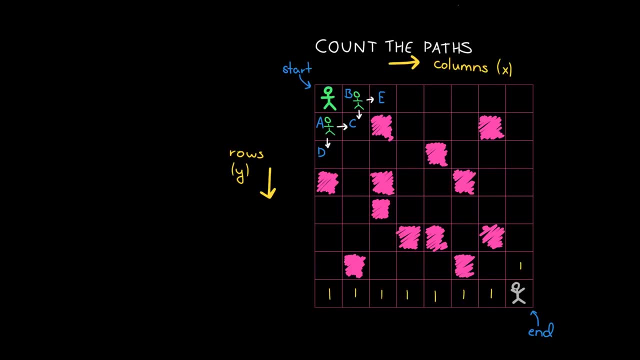 All of these cells have just one path from their cell to the end, which is this path here. Now, what about this cell here? Well, if there's one path going down, one path going to the right, the actual answer is their sum. So there's two paths there. Now, here again, one path there. 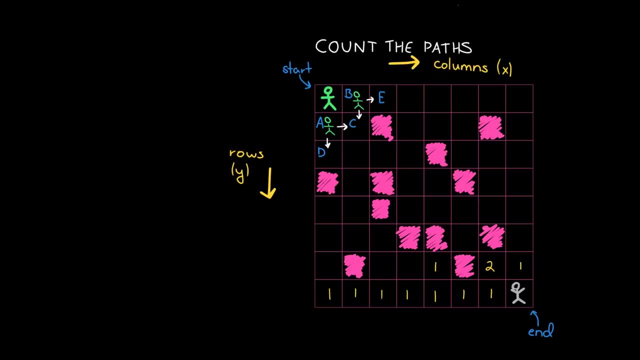 Now, when we go to this cell, there are two paths: going down or to the right. So the sum is going to be these two. this is the sum of those two cells And this one here. well, we can go down or we can. 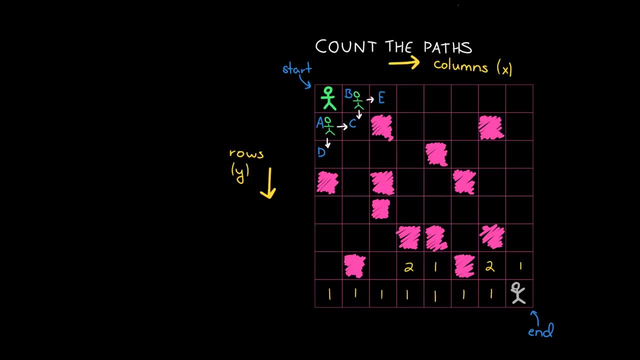 right. There's two paths if we go to the right, one path if we go down. So the actual result for the number of paths from this cell to the end is three paths, And we can double check that if we want. One path is going down and then, all the way over, Another path is going to the right down. 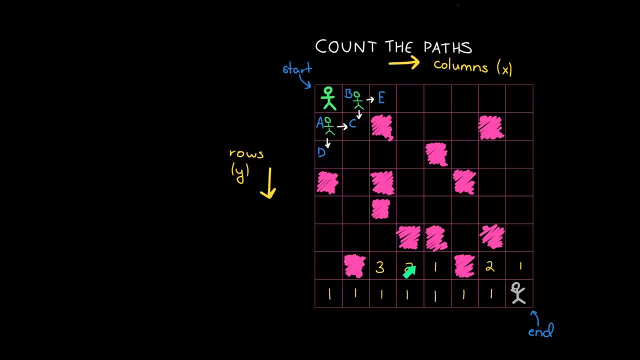 and then all the way over, Or to the right, to the right, again down and all the way over. So sure enough. yes, there are three paths And we can do this exact approach: going through the entire grid, starting from the bottom left, moving to the left, sorry, starting from the bottom right.